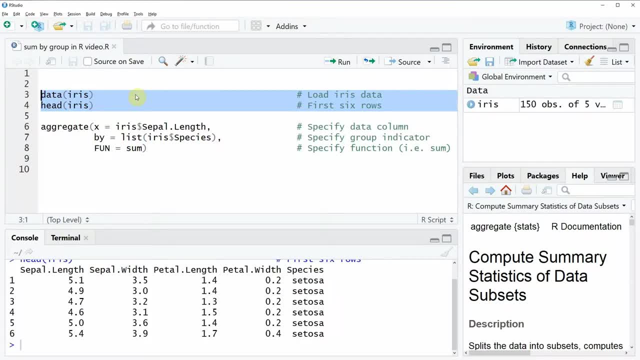 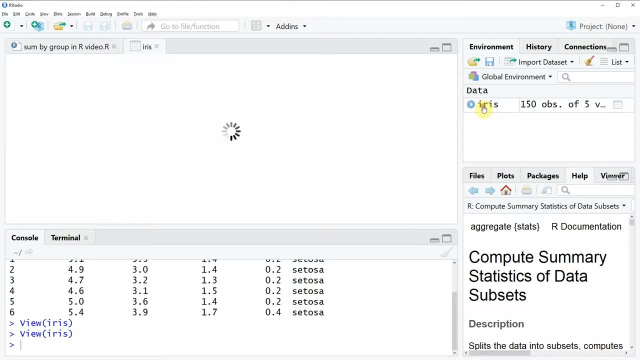 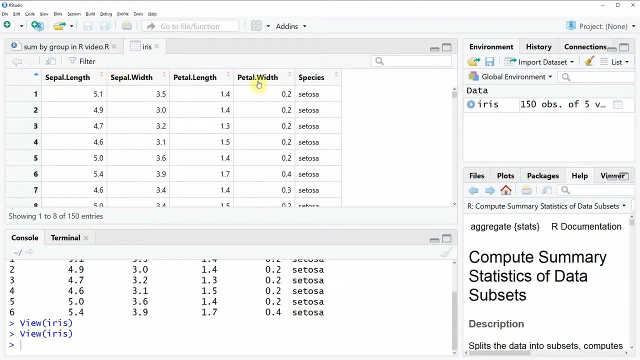 So if you run these two lines of code, you will see that the iris data set appears here at the top right of our R studio. We can also have a look at the data by double clicking on the data and, as you can see, this data set contains four numeric columns as well as a grouping column. 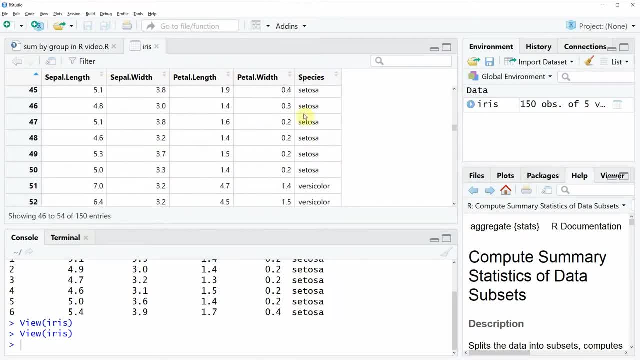 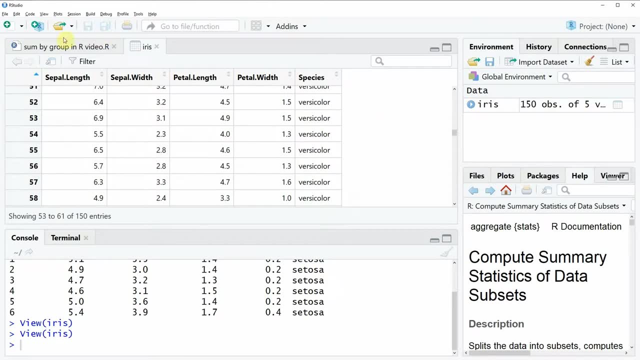 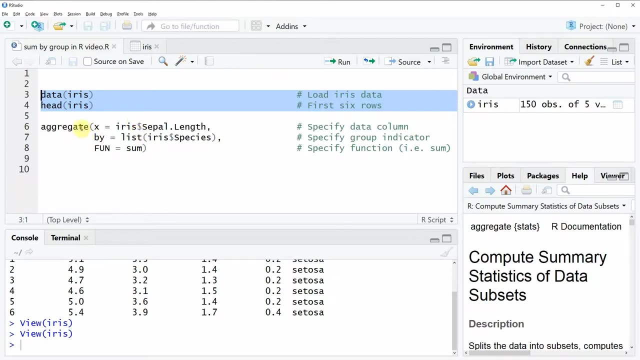 So if you scroll down you can see the first rows are of the group setosa, but then you have also other groups like versicolor and so on. So if we want to compute the sum within each of these groups, we can use the aggregator. So we have the aggregate function, as you can see here in line 6 to 8 of our code. 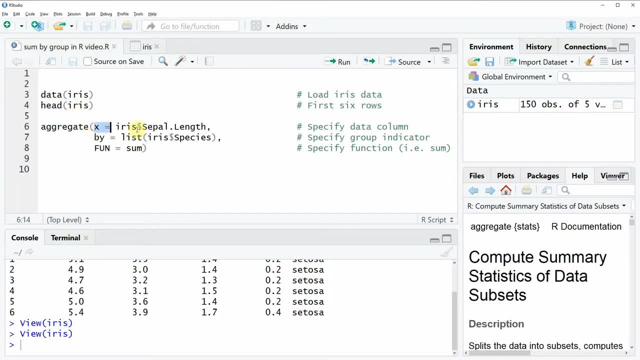 And within the aggregate function we can specify an x value, so a value for which column or vector for which we want to compute the sum by group. So in this case, in this example, we are going to compute the sum of each group of the column sepal length. 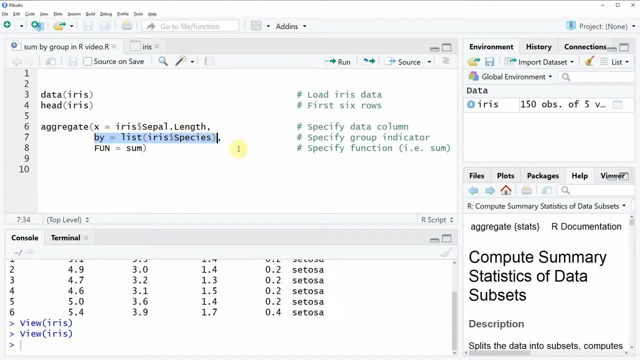 And here, in this example, we are going to compute the sum of each group of the column sepal length. So in the seventh line of the code, in the next line, we are specifying the grouping variable. so in this case we are using the variable species. 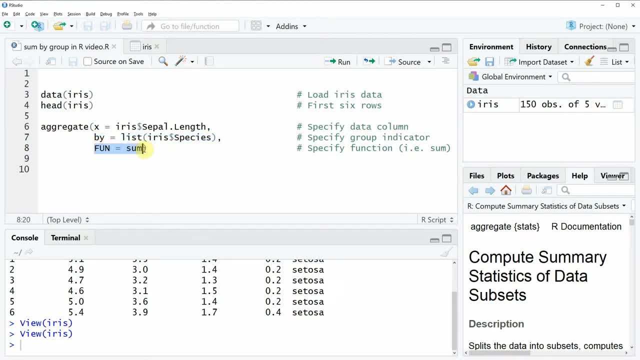 And in the eighth line of code we are specifying the function that we want to apply to each group. So in this case we want to know the sum of each group. so for that reason we are putting here the name of the sum function. Now, if you run this code, 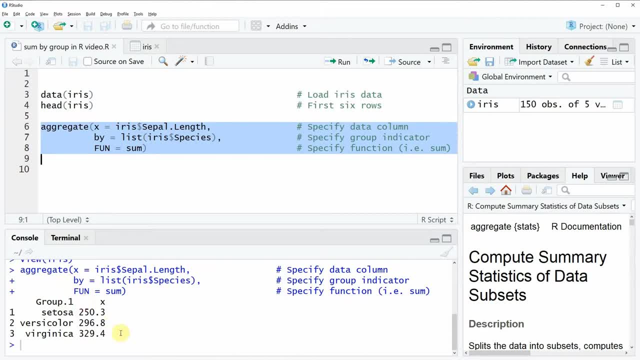 You can see that here at the bottom in the RStudio console, a data table is returned And the data table is showing the sum for each of our groups. So the setosa group has a sum of 250.3.. The versicolor group has a sum of 296.8. 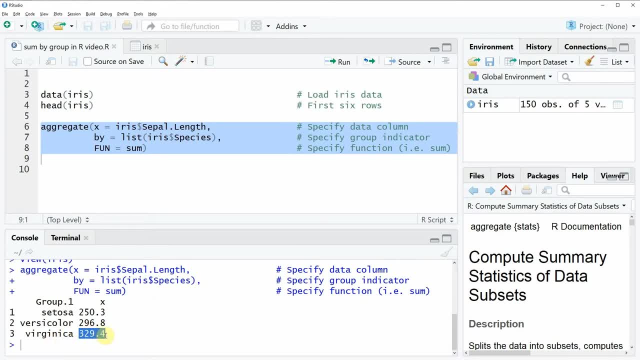 And the virginica group has a sum of 329.4.. Yeah, so that's basically how to compute the sum by group in the R programming language. However, if you want to know more about this topic, you could check out my homepage statisticsglobecom.